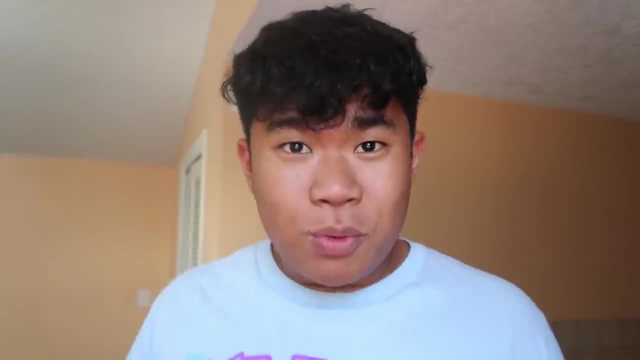 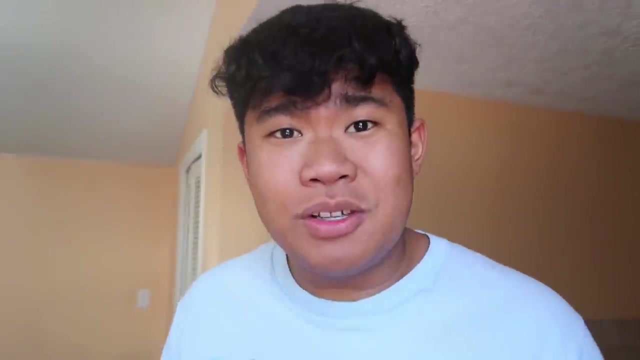 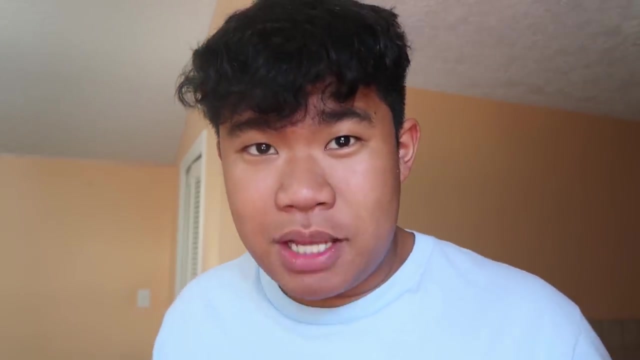 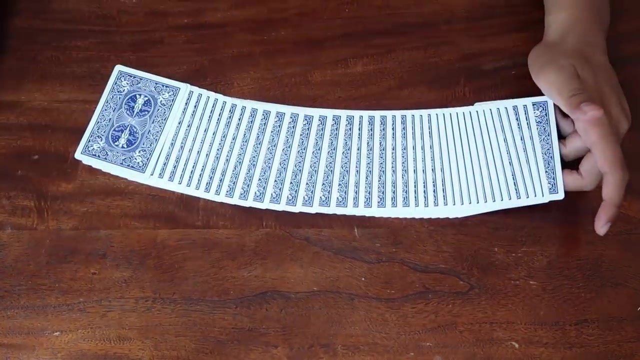 into. it is huge. thank you for 210,000 subscribers. We're growing really, really fast and I just you know I can't thank y'all enough. Y'all really changing my life out here. And thank you for the support on the last video. Y'all absolutely smashed it, One of my favorite videos. If you have not checked it out, it will be linked at the top of the description. Not a magic video, It's me surprising one of my best friends with a laptop. so go peep that. But anyways, enough talking, Let's teach you the easiest, most self-working card trick. So here is the performance on one of the world's easiest card tricks that are gonna fool your friends and family. This is a. 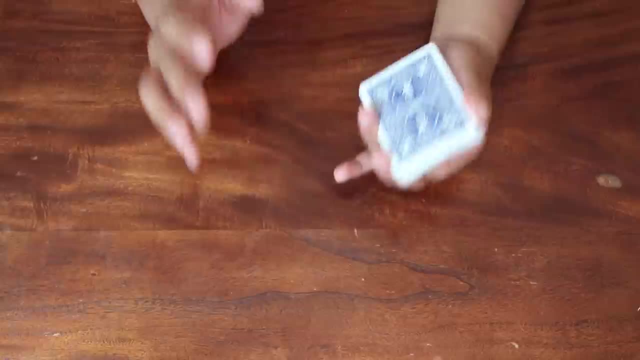 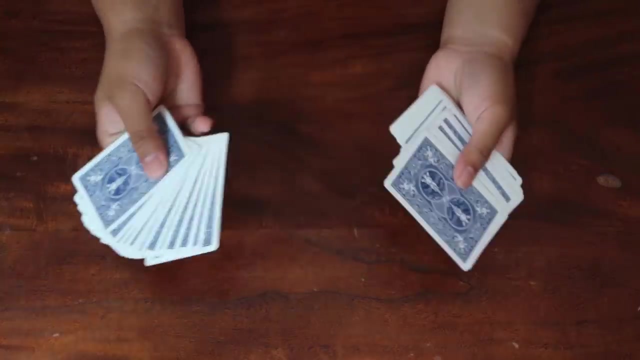 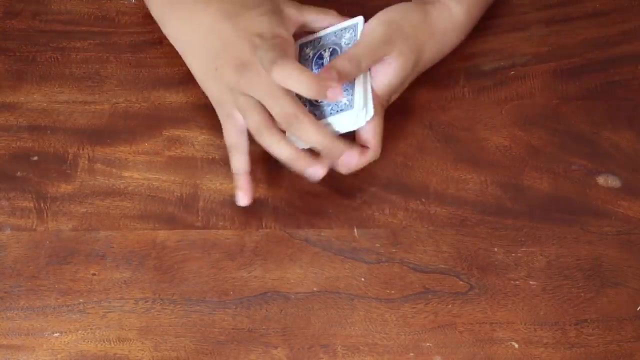 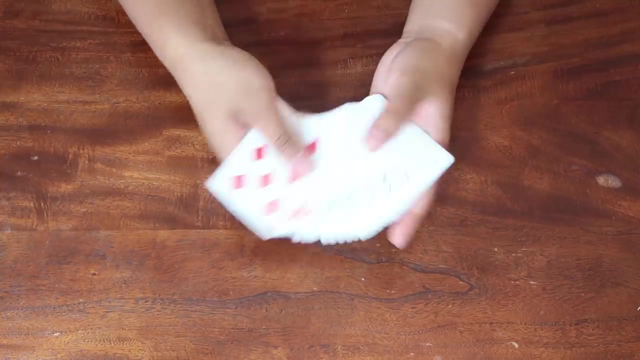 self-working card trick. This is a self-working card trick. You literally don't need any skill. This is so easy. You could do it. Your mom could do it, Your grandma, your grandpa- Heck, my dog could probably do this magic trick. I don't even have a dog, so like, that's literally how easy it is. So, yeah, let's get into the performance. So for this we need a deck of cards. of course, We're gonna give it a nice shuffle, give it a nice little mix, so you know that it is truly a normal deck of cards. You can see all the cards are mixed like. so Okay, what we're gonna do is I'm gonna take the deck and I would ask you to 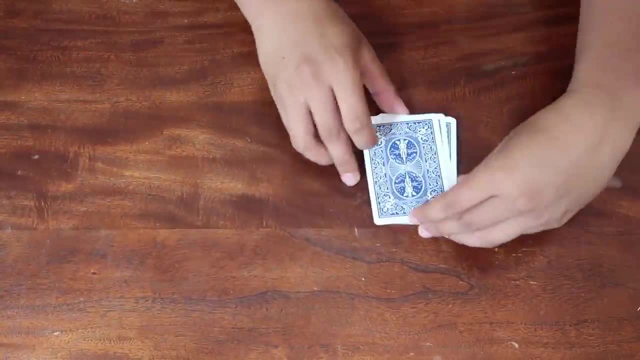 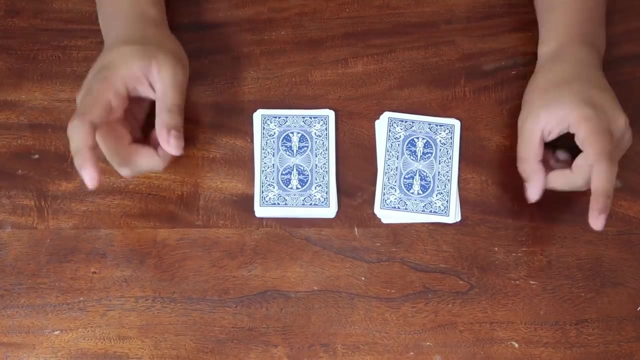 go ahead and cut the cards. Now, obviously you're not here so you can't cut the cards. so I'm gonna do it for you. but you would typically have someone just cut the cards. So they cut the cards roughly in half and then you tell the person: do it one more time. Go ahead and cut each pile. 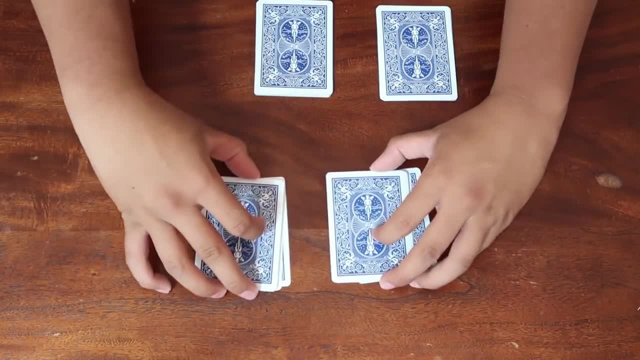 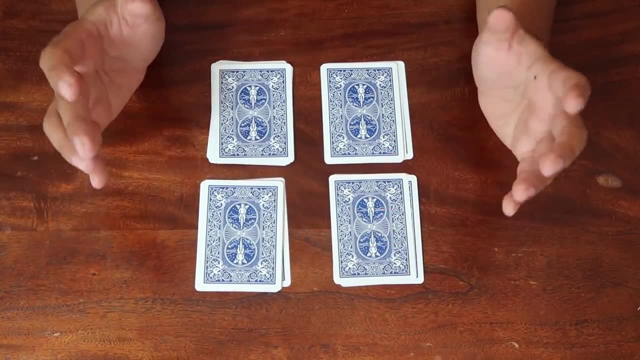 in half again. Now we should have four beautiful piles just like. so I'll move them over here and we're gonna do a little bit of a magic formula to magically make something happen. Check it out, Watch. This is the magic formula. 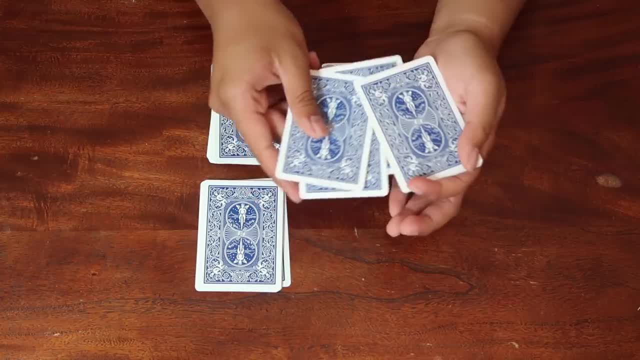 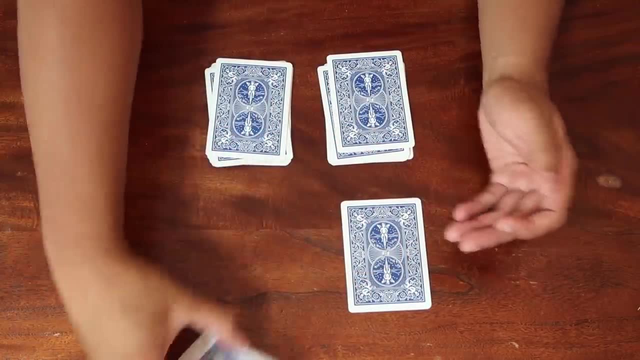 All you gotta do is take three cards off the top of the deck of each pile, put it to the bottom, and then take a card and place it on top of each stack. so you do that with every pile. look at this: if you take three cards, you put it to the bottom. you take. 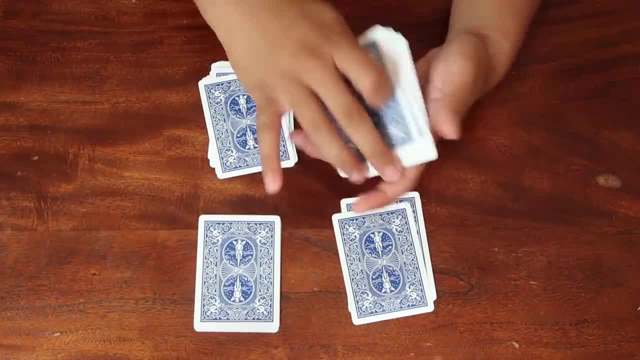 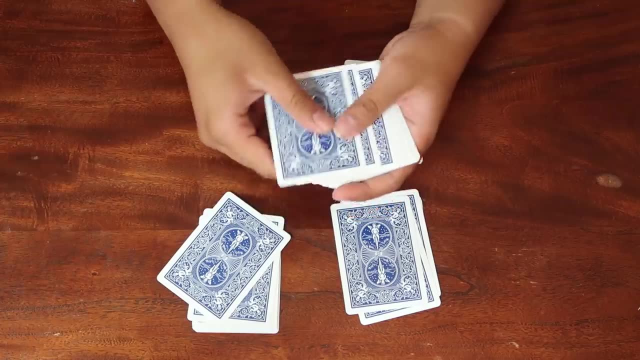 one card each on each stack and you repeat this with every single stack. now this one- three cards- goes to the bottom, one card on each pile, and then the last pile- right here- three cards- goes to the bottom, and then there is one card on each pile. now it may not seem like we did anything crazy. 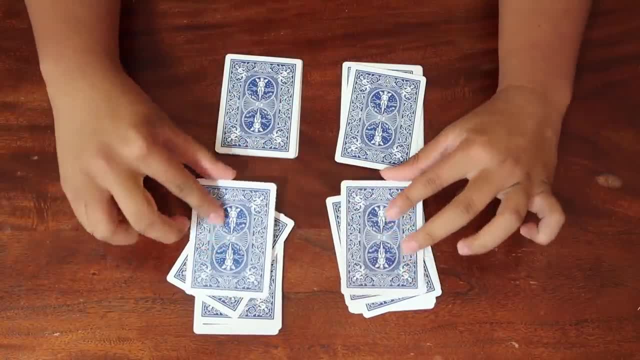 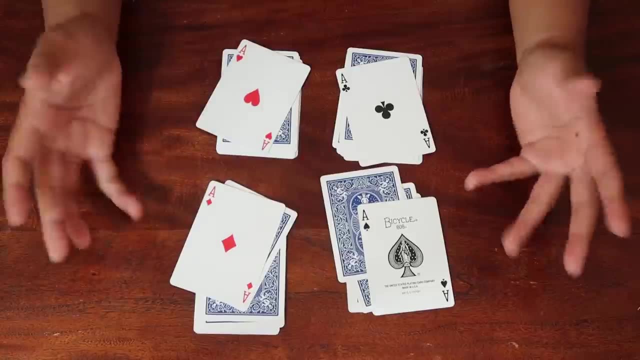 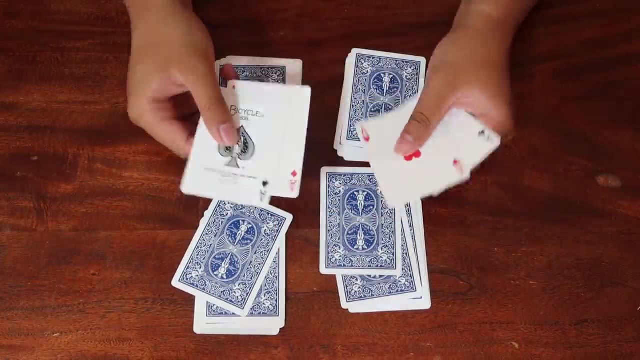 but look, I'm a magician. I have to do is wave, snap. that magical formula has now made it so that every single card on the top of the stack is the aces- just like that. isn't that freaking cool? and, believe it or not, you could do this right now with literally no skill, if you've never touched a. 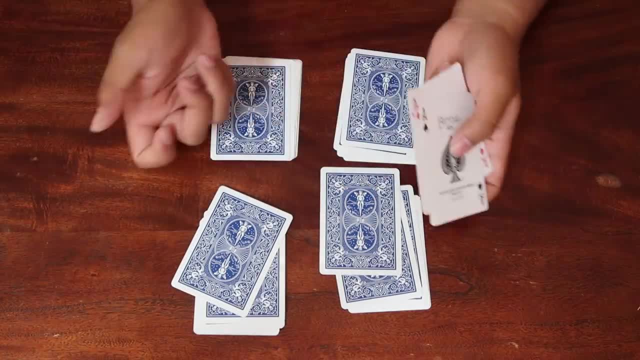 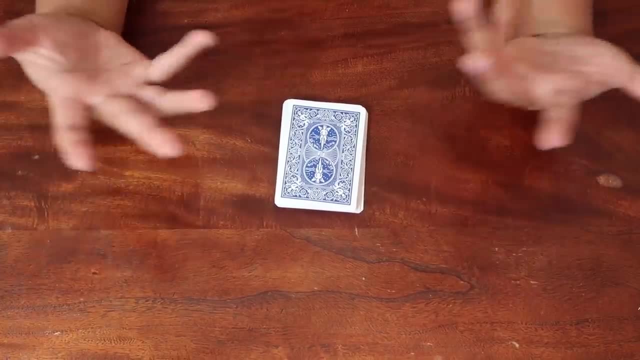 deck of cards in your life. you could do this right now. let's get right into the tutorial. so to do this, all you do is you take the four aces and you put it on top. done, anyways, that is it. that's literally all you do, and you're. 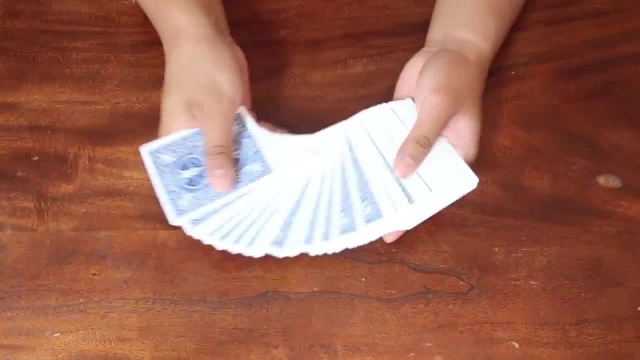 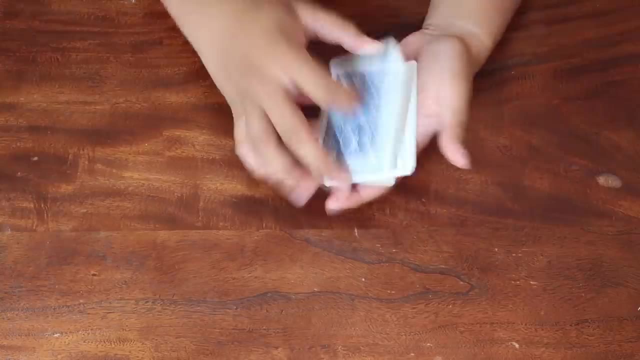 pretty much done with the trick. there's a few more things you got to do, but, like, that's basically it. you just got to set it up with the four aces on top of the deck. what I like to do is I like to shuffle the cards. how I show the cards make sure is that it stays on top. I do this through a series. 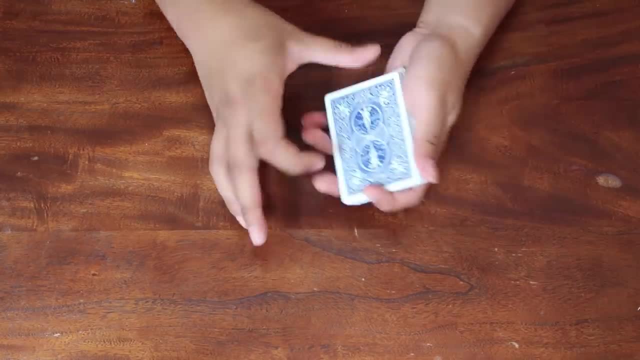 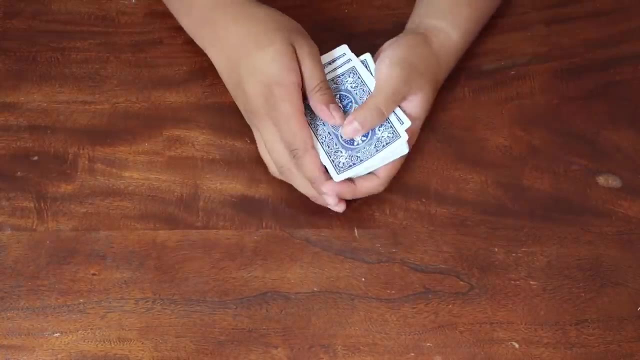 of false shuffles, so it might look like I'm mixing up the cards, but in reality I'm not. if you want a tutorial on fake shuffles, I have one coming soon. or you can look one up on YouTube. literally just search up the phrase false shuffle and you just search it up and like how to do a false shuffle. 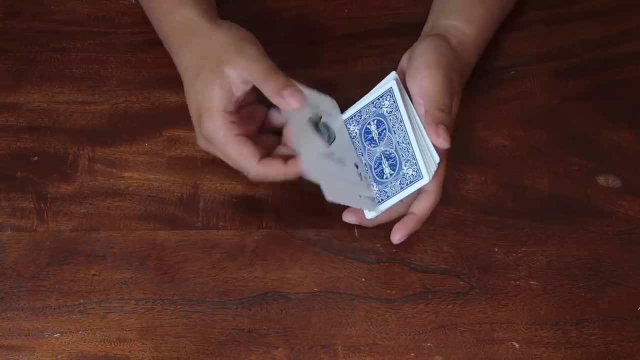 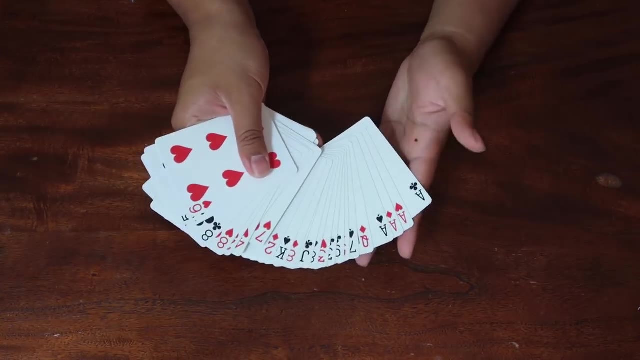 you should be able to find it. so yeah, I start off with this. with the four aces on top, you don't need to shuffle the cards. you could literally just say, hey, look, it's all mixed up, and then you just don't show the end where all 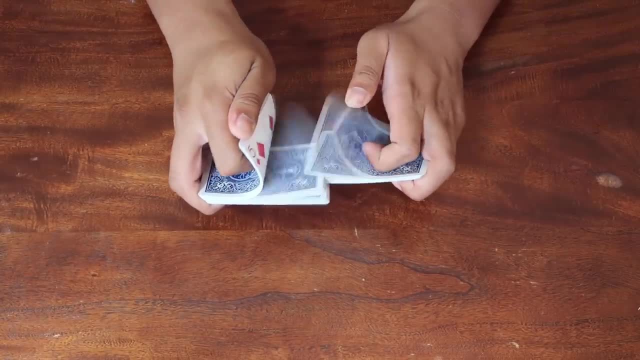 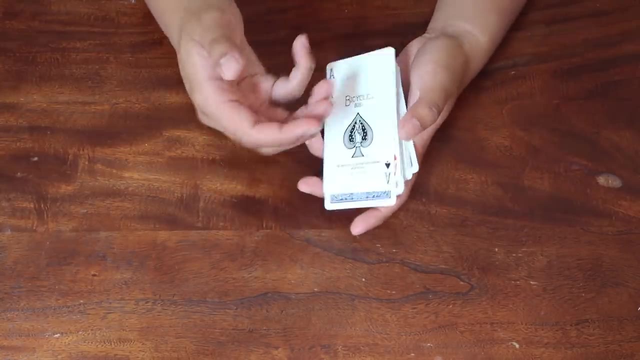 the aces are. but just to convince people even more, I shuffle it, keeping the aces on top, and of course I do some fake mixes and cuts to make sure that they stay on top. this is just more advanced stuff. you don't have to do this again. this is supposedly just a trick that you can do. 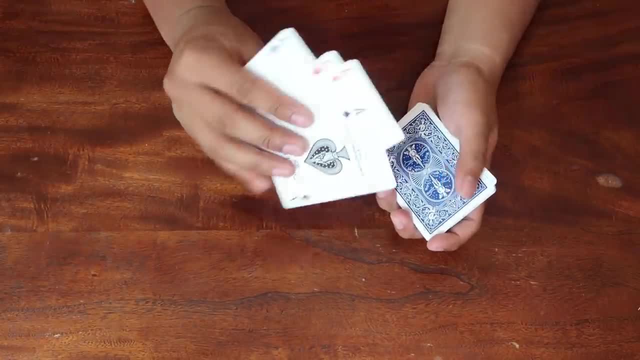 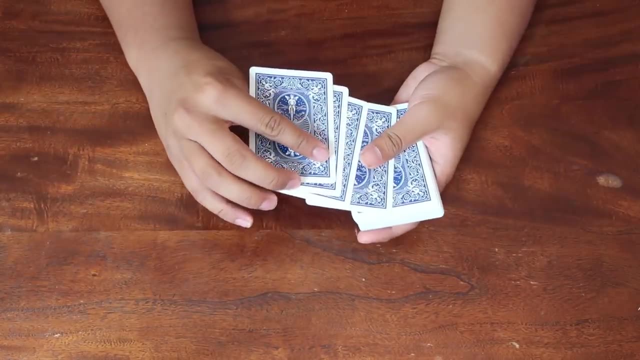 on with no skill. so if you literally want to just keep the four aces on top- and you can your trick- you can even just show the other cards that they're mixed. so once you're in this position, you're basically done. you literally tell the spectator to. 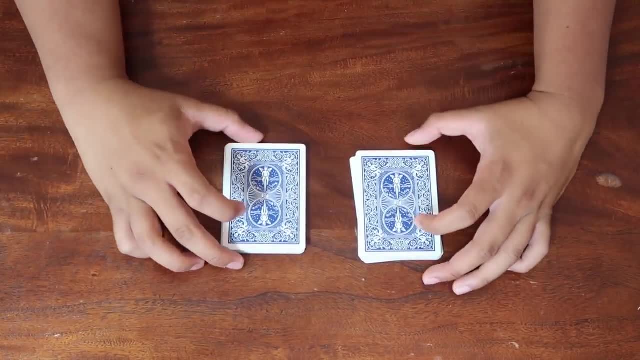 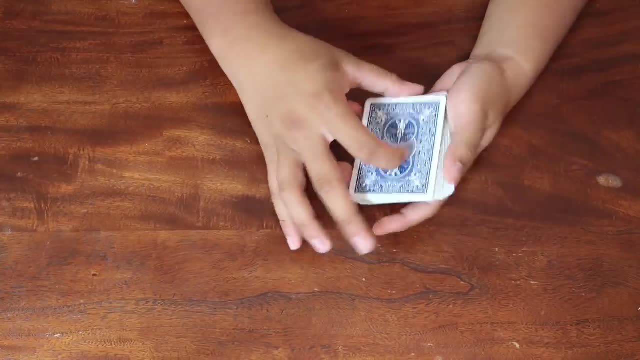 cut the cards. that will cut the cards in half, and then you're gonna cut the cards again. now, the only thing you need to do while you're doing this is you need to keep track of where the aces are. so the aces are on the top right now, when you. 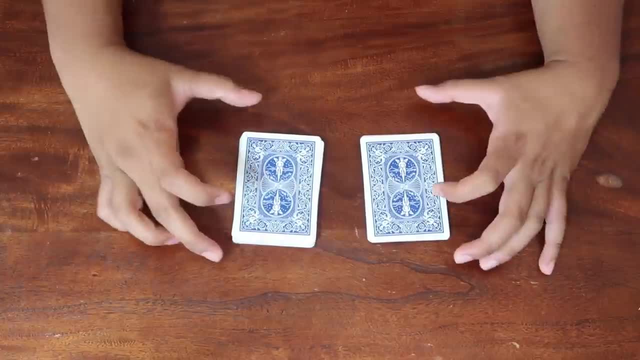 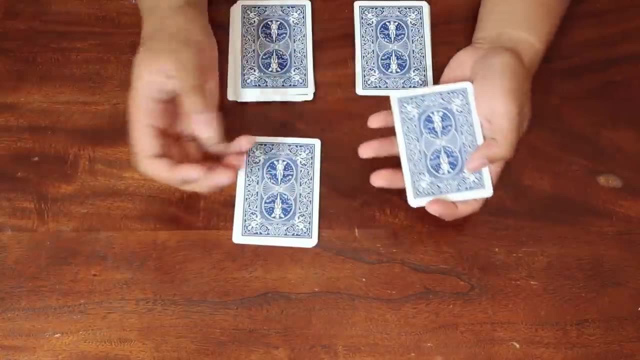 have them cut the cards, now the aces are here, and when you have them cut it again. now the aces are here and all you have to do is follow where the aces are. once you know what stack it's at, literally all you're gonna do is you're gonna make.